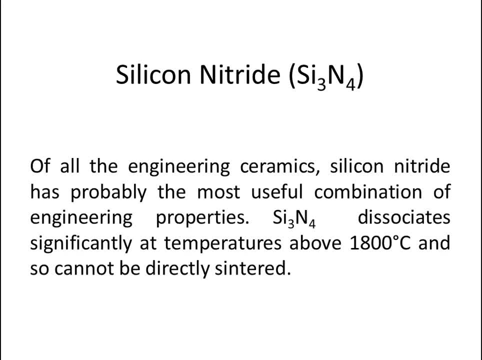 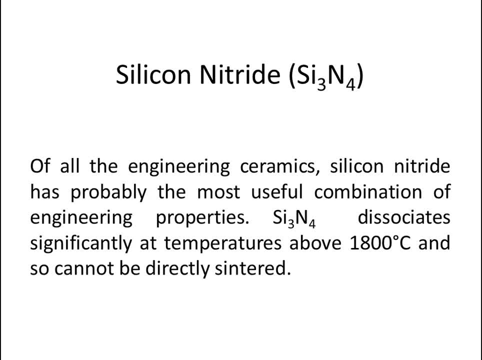 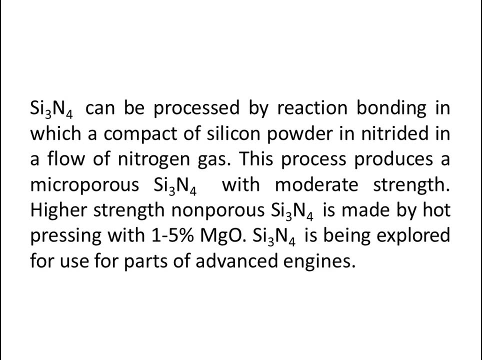 of engineering properties. Silicon nitride dissociates significantly at temperatures above 1800 degree celsius and so cannot be directly sintered. Silicon nitride can be processed by reaction bonding in which a compact of silicon powder is nitrided in a сilicone compound. 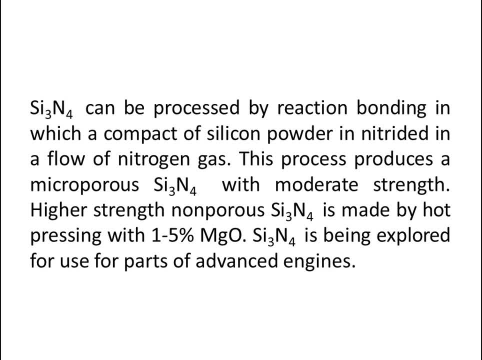 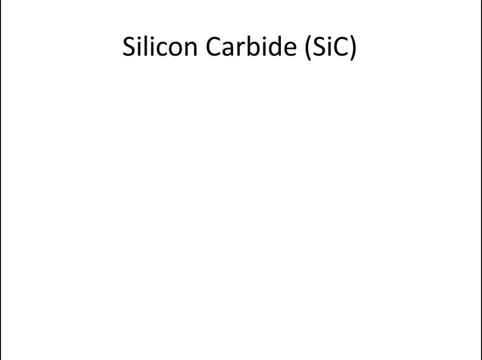 flow of nitrogen gas. this process produces a micro porous silicon nitrite with moderate strength. higher strength, non-porous silicon nitrite is made by hot pressing with one to five percent magnesium oxide. silicon nitrite is being explored for use for parts of advanced engines. now let's talk about silicon carbide. 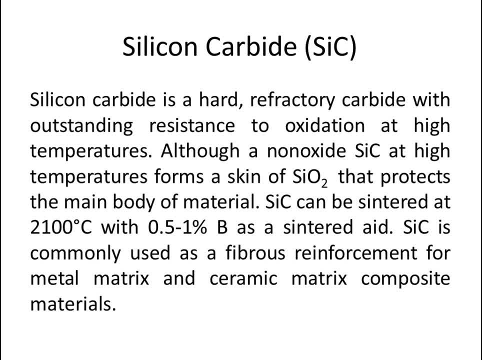 silicon carbide is a hard refractory carbide with outstanding resistance to oxidation at high temperatures. although a non-oxide silicon carbide at high temperatures forms a skin of silicon oxide that protects the main body of material, silicon carbide can be sintered at 2100 degrees celsius. 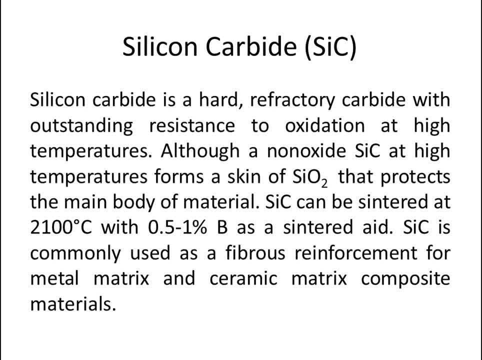 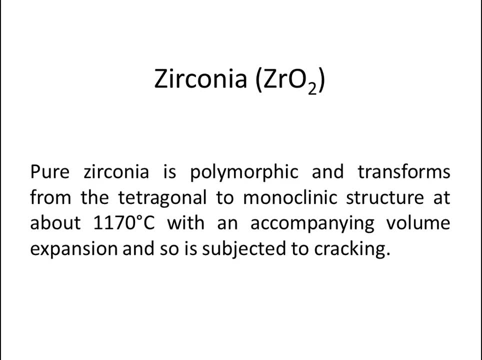 with 0.5 to 100 degrees celsius percent boron as sintered aid. silicon carbide is commonly used as a fibrous reinforcement for metal matrix and ceramic matrix composite materials. now let's talk about zirconia. pure zirconia is polymorphic and transforms from the tetragonal to monoclinic structure. 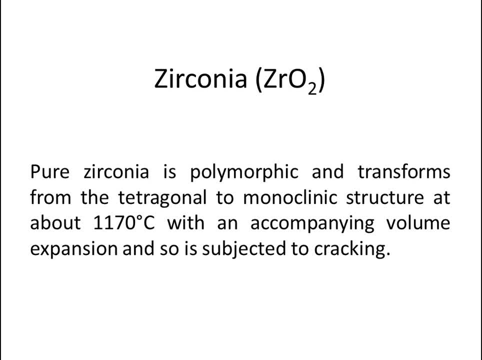 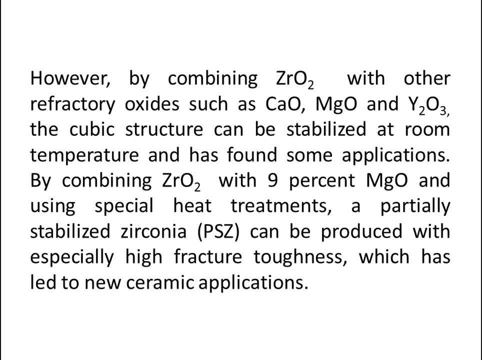 at about 1170 degrees celsius with an echo accompanying volume expansion, and so is subjected to cracking. however, by combining zirconium oxide with other refractory oxides, such as calcium oxide, magnesium oxide and other oxide, the cubic structure can be stabilized at room temperature and has found some applications. 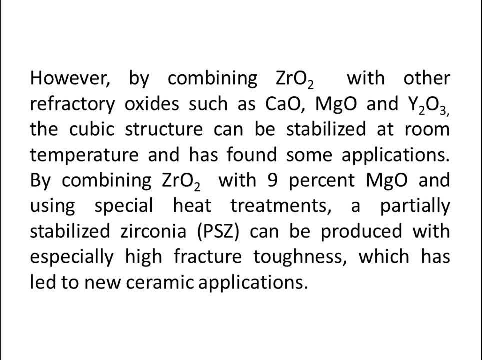 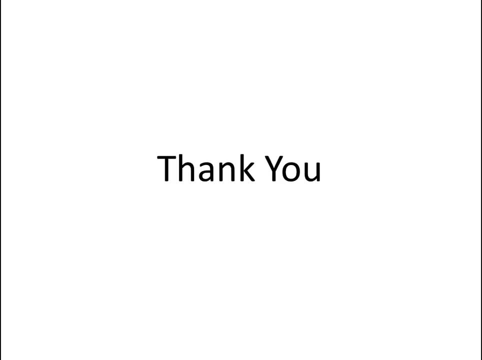 by combining zirconium oxide with nine percent magnesium oxide and using special heat treatments. a partially stabilized zirconia can be stabilized at room temperature with an echo, accompanying volume, expansion and so on. as a consequence, the surface can get cracked, produced with specially high fracture toughness, which has led to new ceramic applications.